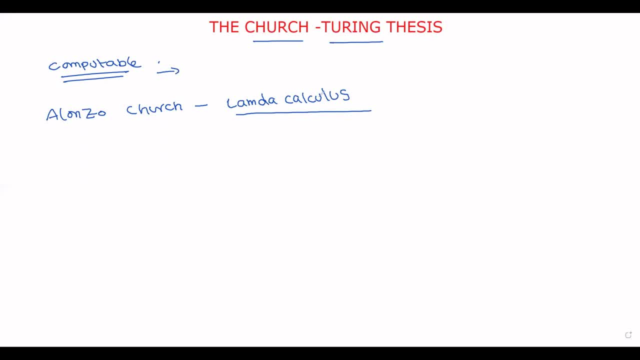 or a language Mathematical calculation. If it is calculated by using this Lambda Calculus, that thing is called computable. Later on the scientist Alan Turing developed a mission called Turing Mission. So he said that anything that is calculated or computed by using Turing Mission. 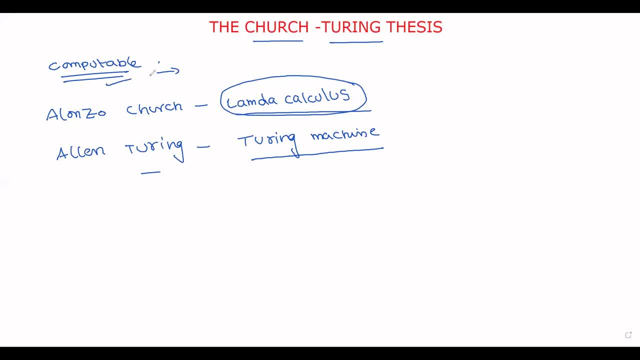 is called computable. So two different Scientists give two different meanings And before going to this one, which one is the correct one? That is, either Lambda Calculus is the correct one or Turing Mission is the correct one. Before going to this one, we have to know different variants of Turing. 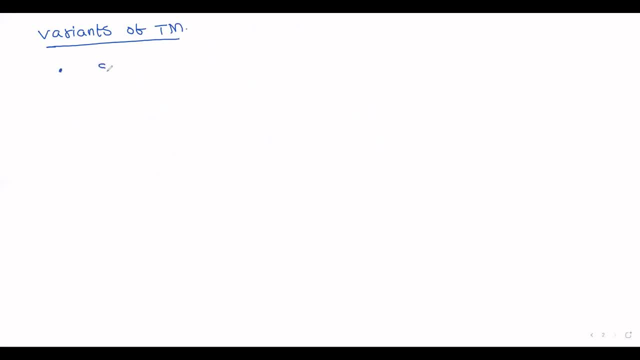 Mission. Up to now, we discussed a single tape Turing Mission And remember, we have not only a single tape Turing Mission, We have many tape Turing Mission. That means multi-tape Turing Mission is also available. That means, instead of using single table, the input is written on multiple number of. 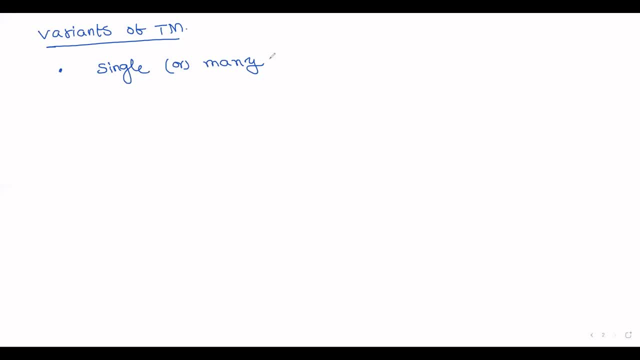 tables and the automata at a time implement all the tables. This is one variation And infinite on both ends. That means we up to now we know we are constructing a Turing Mission. Generally the length of the Turing Machine is infinite, But we generally write our string from the starting of the tape. 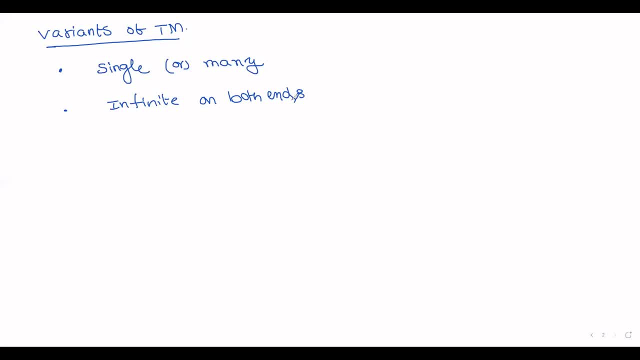 And the right side is the only infinite length. But we have one more variation that is infinite on both the ends. Now alphabets only. That is 0,, 1 or more. That is, a Turing Mission can accept Only the alphabets. 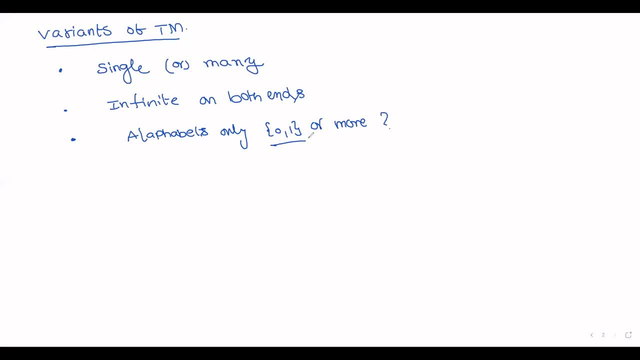 0 comma 1 or at a time, there is a chance to accept more number of alphabets, and is it possible to allow non-determinism, that is, a non-deterministic Turing mission, non-deterministic Turing mission. these are the different variations. then what is the relation of this thing to the Turing mission?